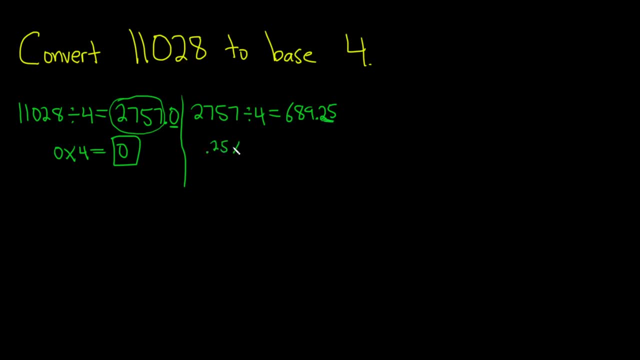 you take this number and multiply it by 4.. 0.25 times 4, 0.25 times 4,, which is 1.. So the remainder is 1.. Okay, the remainder will always be 0, 1,, 0,, 1, 2 or 3 in this problem. 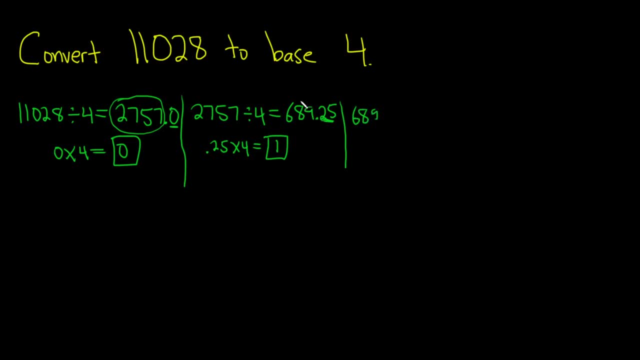 So let's do it again. Let me take 6,, 8,, 9. So take this one and divide it by 4. So basically, you just keep taking the whole number part and dividing by 4. And you stop when this part is 0. So that will happen at some point, Let's see. So this: 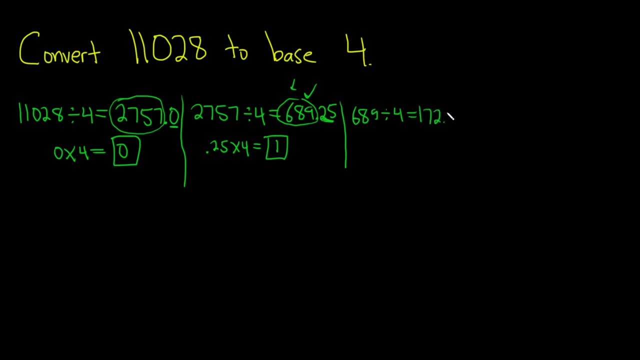 is 172.25.. So now you take this part and multiply it by 4.. And so we get 1.. Then you do it again: Take this part, 172,, divide it by 4.. 172, divide it by 4.. So this is, let's see what. 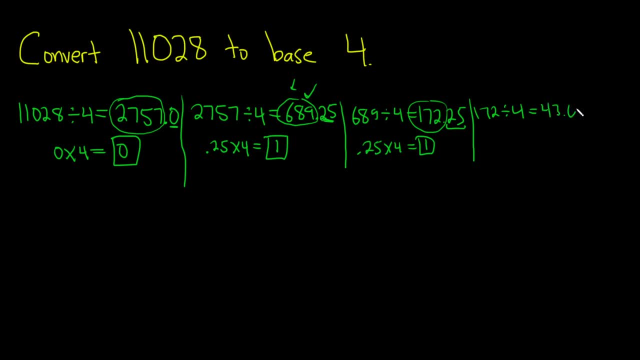 we get 0.0.. So the remainder is 0. But again, if you wanted to follow the steps, you would just do this and you'd get 0. Then you do it again, except you take 43. So 43 divided. 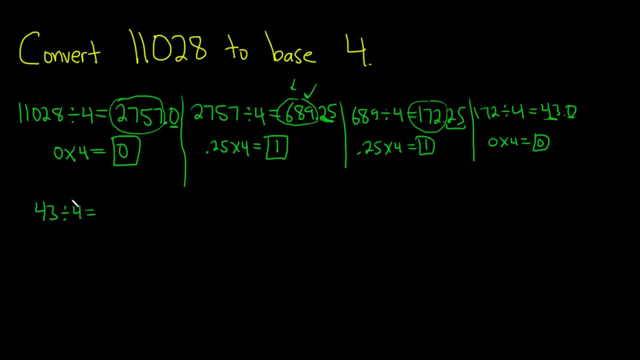 by 4.. So this is 10.75.. You know you could do some of this in your head too. Like you know, 43, 4 goes into 43 10 times and 3 is left over. So the remainder is 3.. But this: 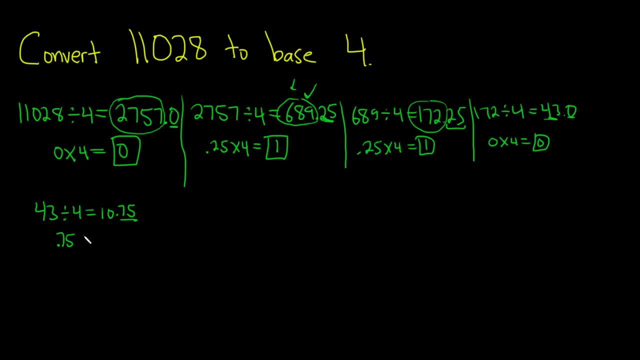 is just a way So you can write it down and just like follow the steps so that you can always get it right, Because sometimes it's hard to do in your head right. So see 3.. Then you go to the 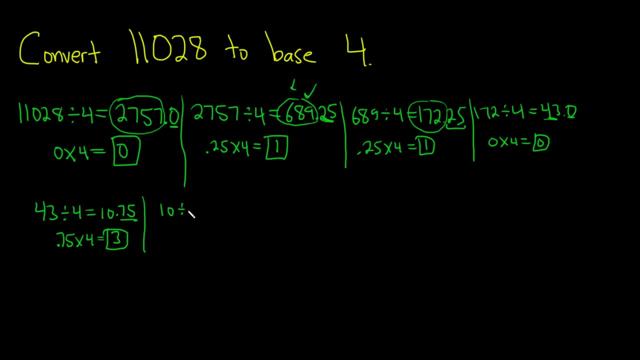 next one: 10.. 10 divided by 4.. This time the remainder should be 2, right, 4 goes into 10 twice and you have 2 left over. But let's work it out. Let's see 10 divided by 4.. I. 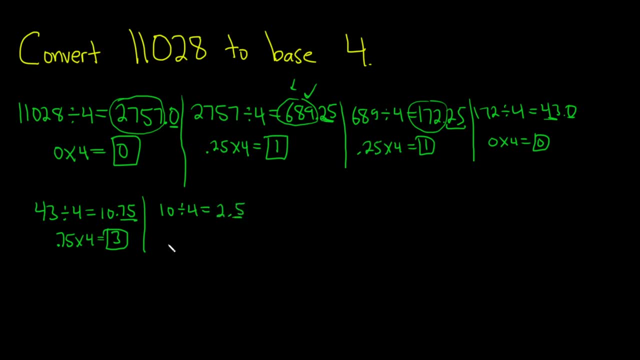 got 2.5.. Then you take the decimal, So 0.5.. Multiply it by 4.. Which is which is 2.. Then you do it again: 2 divided by 4.. Right, take this number divided.